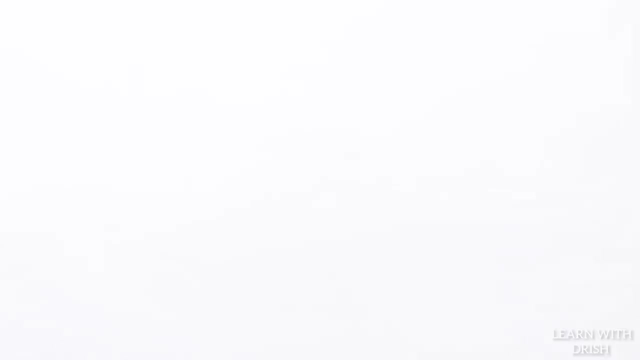 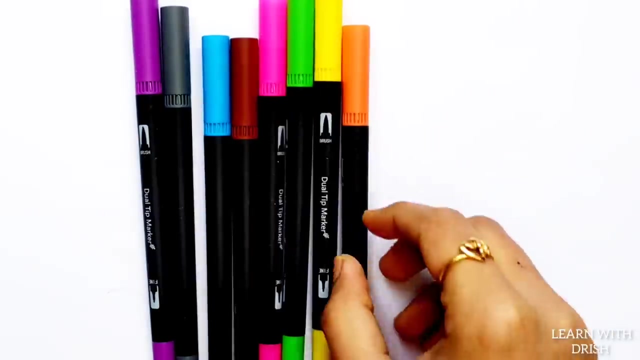 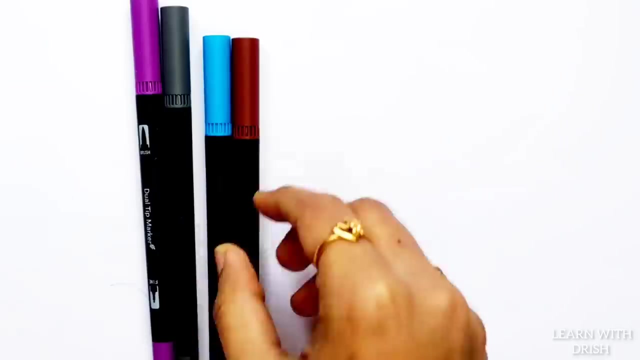 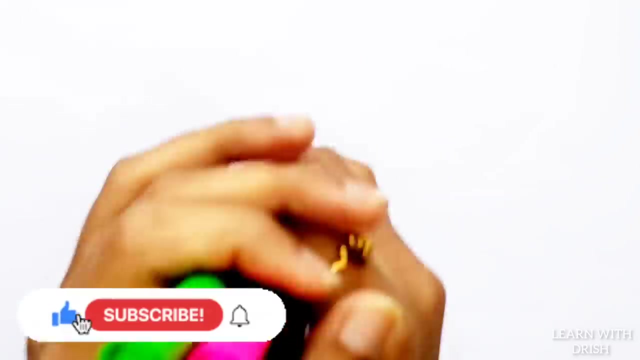 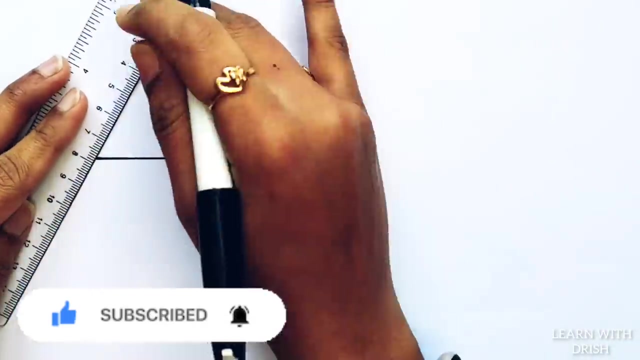 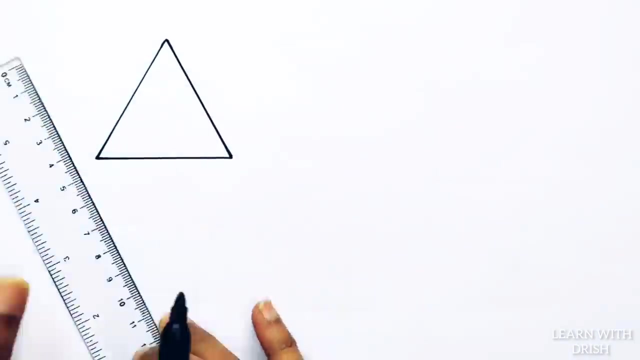 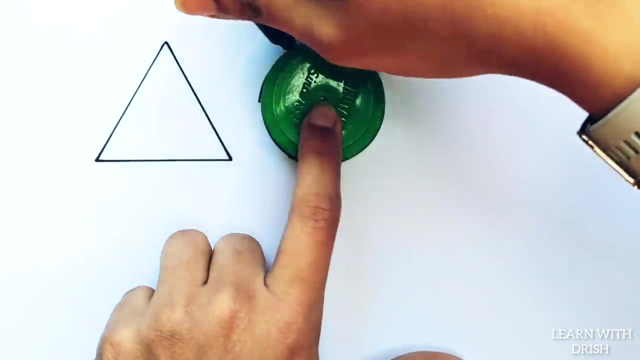 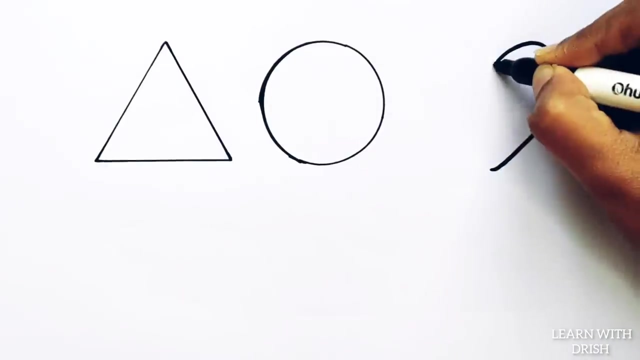 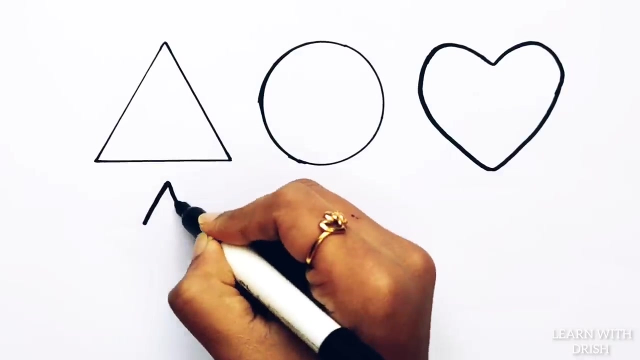 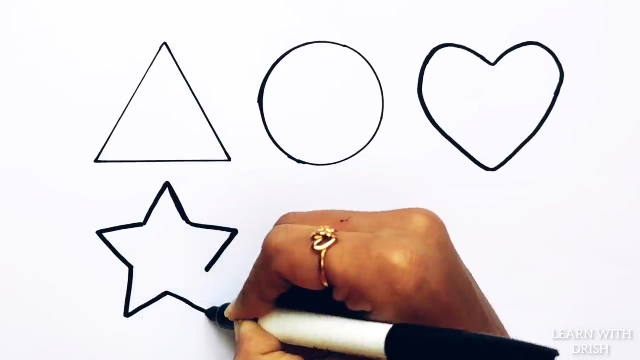 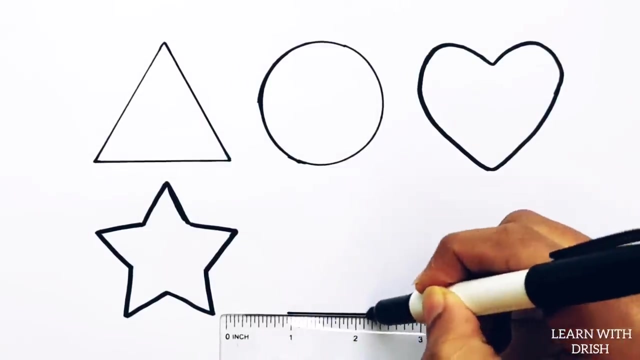 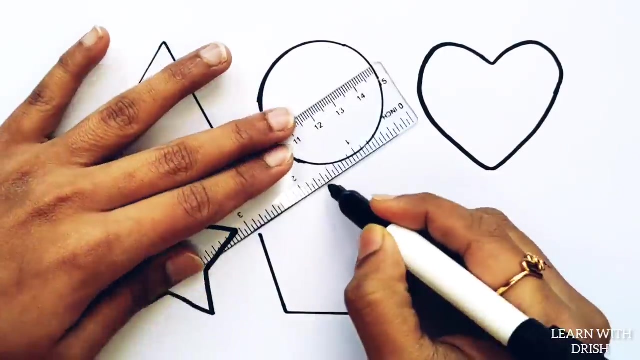 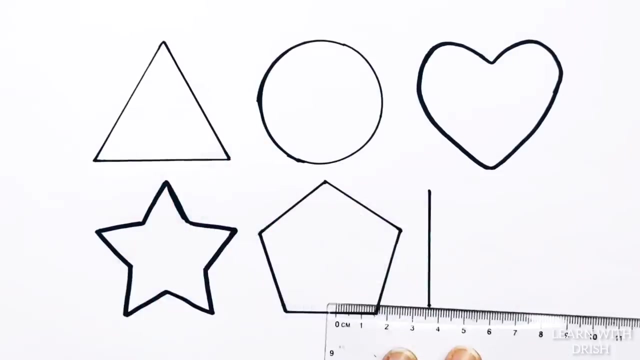 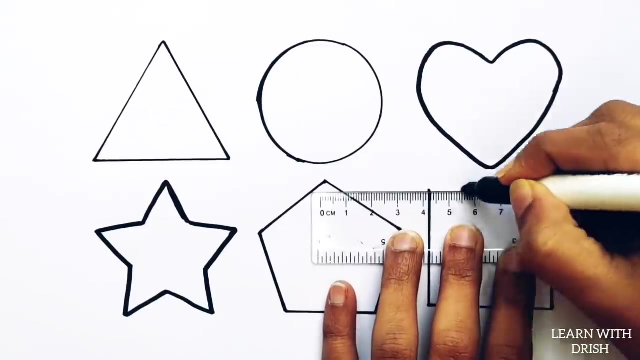 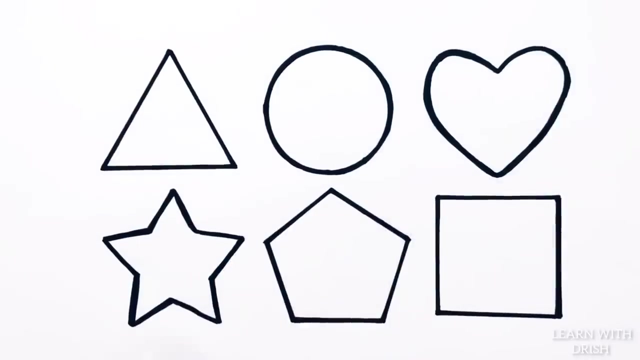 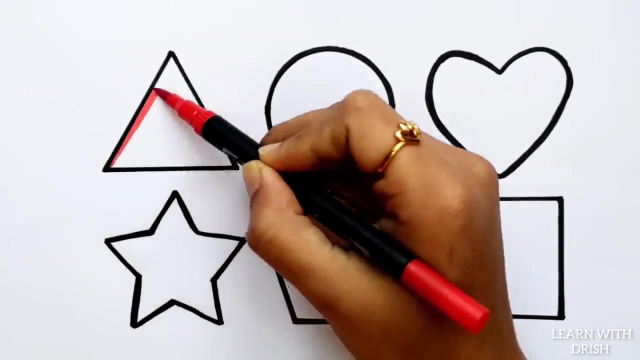 Hello, red colour, orange colour, yellow colour, green colour, pink colour, brown colour, blue colour, grey colour, purple colour. Triangle Circle Heart- PENTAGON- PENTAGON SQUARE. TRIANGLE CIRCLE- HEART STAR- PENTAGON- SQUARE. 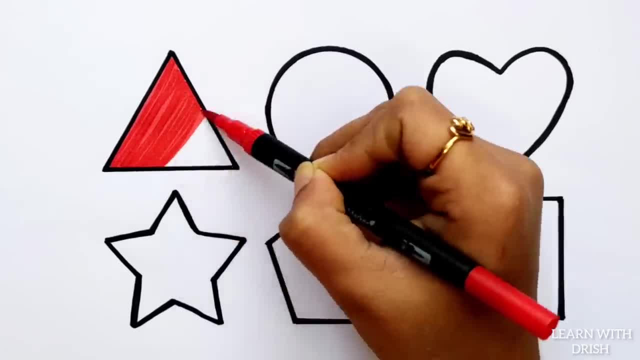 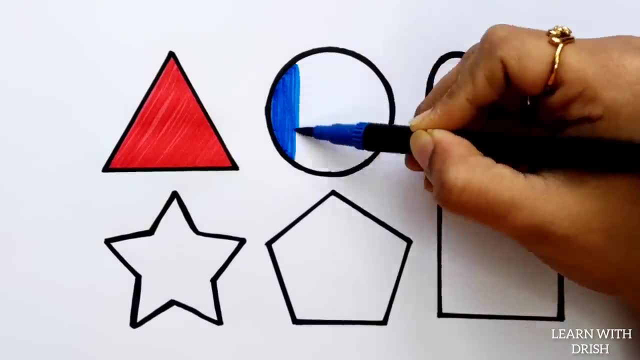 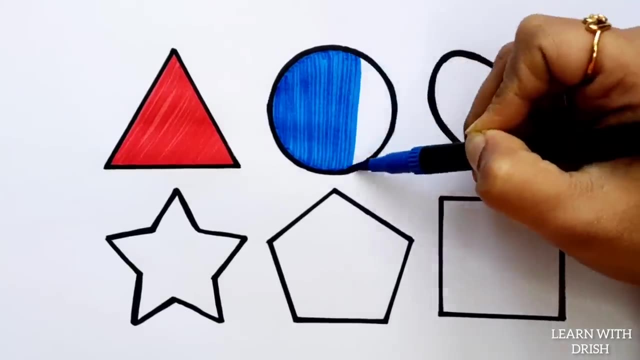 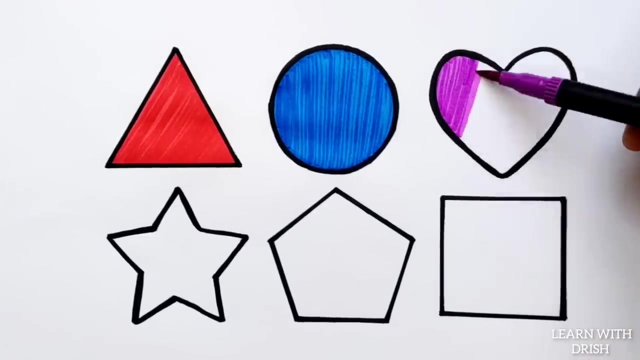 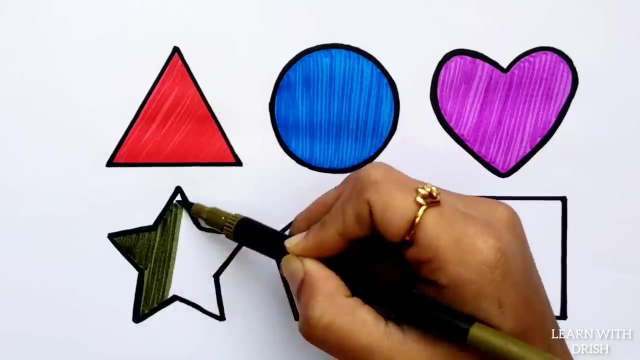 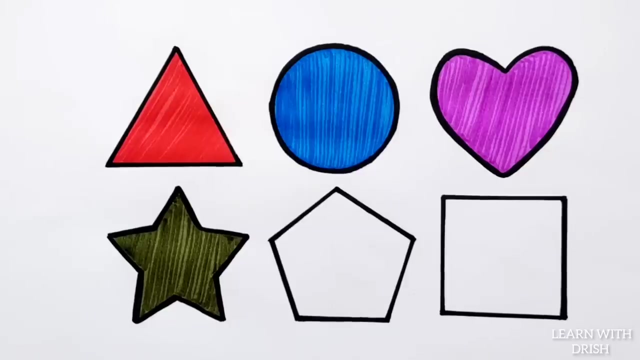 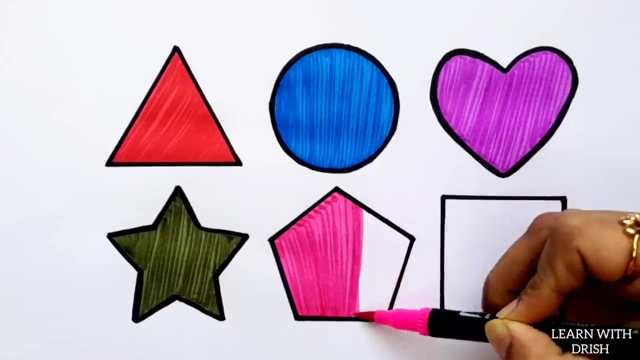 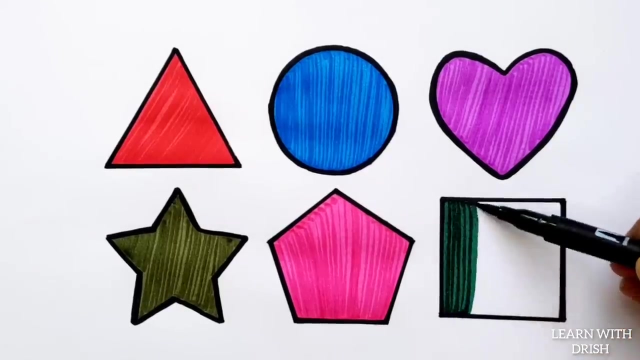 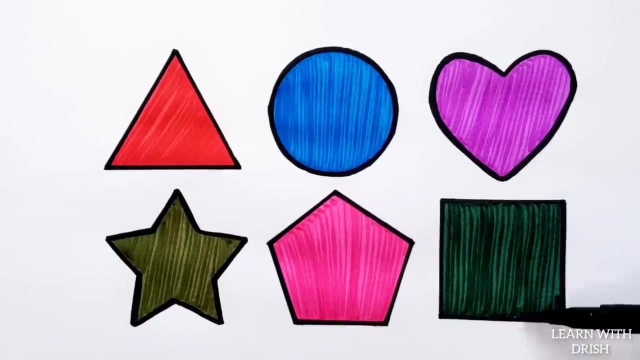 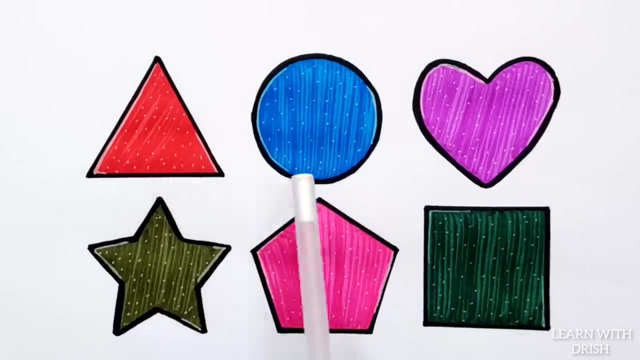 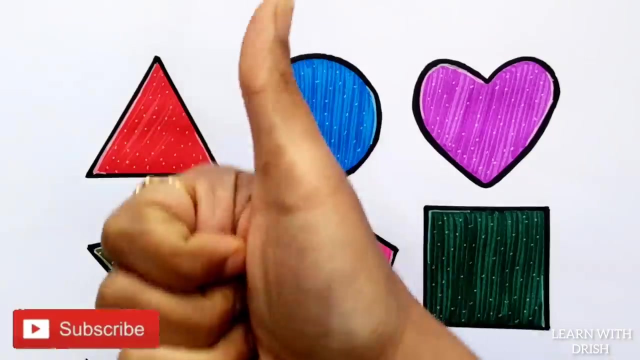 RED COLOUR- PENTAGON. DARK BLUE COLOUR. DARK BLUE COLOUR. PURPLE COLOUR. Olive green colour. Pink colour- Dark Green colour- triangle: circle- heart star- pentagon square. thank you so much for watching. don't forget to like and subscribe. see you next video. bye.